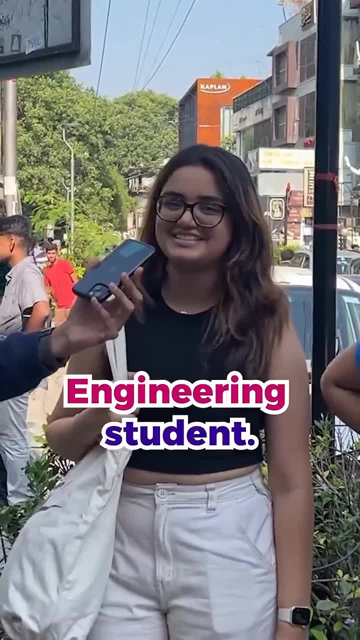 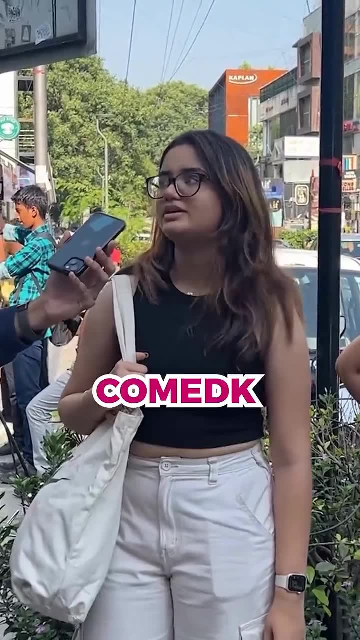 What do you guys do? I'm a second year artificial intelligence and data science engineering student. How did you guys get into this? I wrote COMET-K and CET exams and I got in through the last round of COMET-K. So like now, since AI is taking over everything, right? 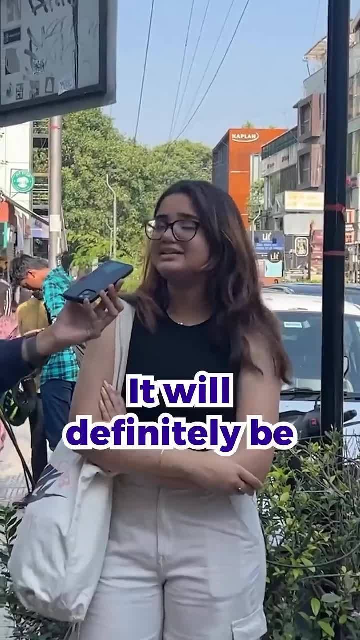 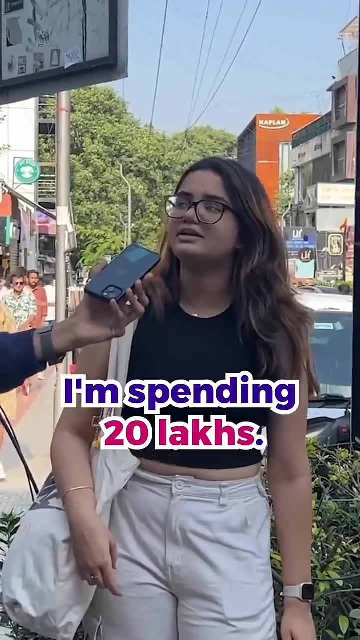 Is that an advantage for your degree or is that a disadvantage For my degree? it will be definitely an advantage because I'll be training the models and working with it. How much did you guys spend on your degrees? I'm spending 20 lakhs. 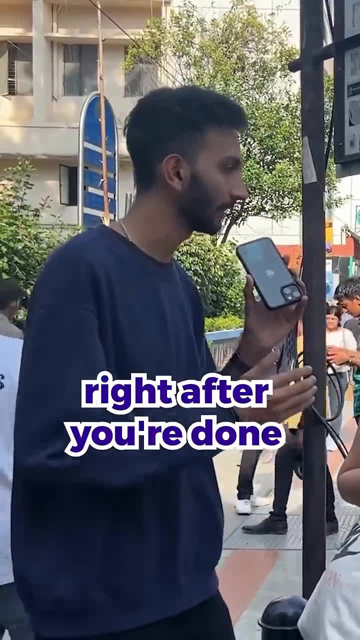 So why don't you tell us how the starting salary looks right after you're done with your degree From my college? it will be around 4-5 lakhs. 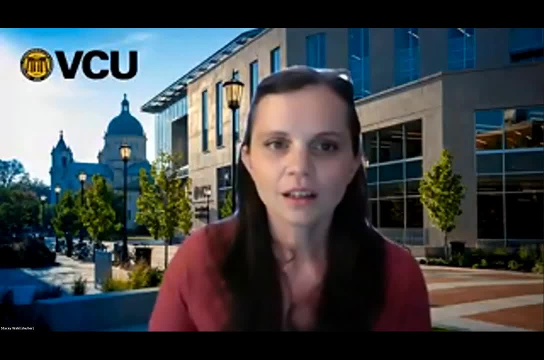 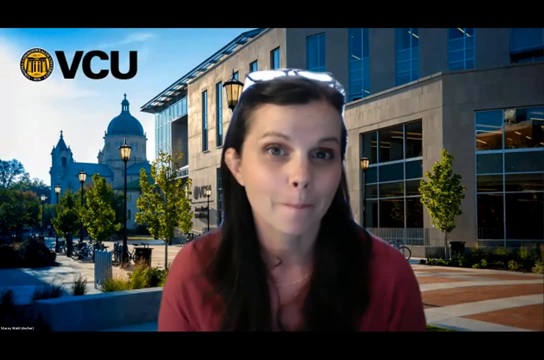 Okay, so hello and welcome. This is the How to Talks by Postdocs, and today we have Dr Cobley, who's going to be talking to us about Bayesian statistics. Dr Cobley is an Aracta Research Fellow in Jason Reed's lab in the physics department here at VCU. He is researching 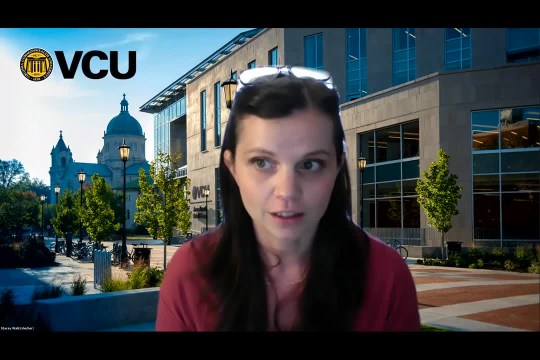 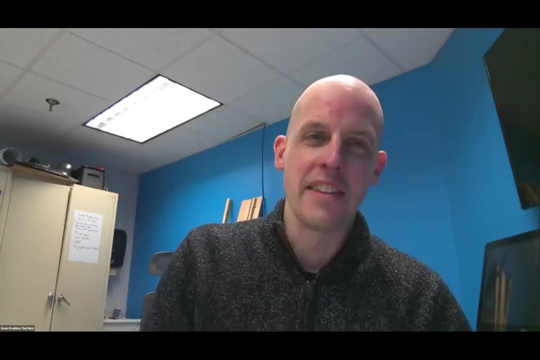 a novel method for detecting genetic mutations using biophysics. Formerly, he taught middle school mathematics in Boston and DC before earning his PhD in applied science from the College of William & Mary. Let's welcome Dr Cobley, and here we go. Hi, everybody, and thanks Stacey. 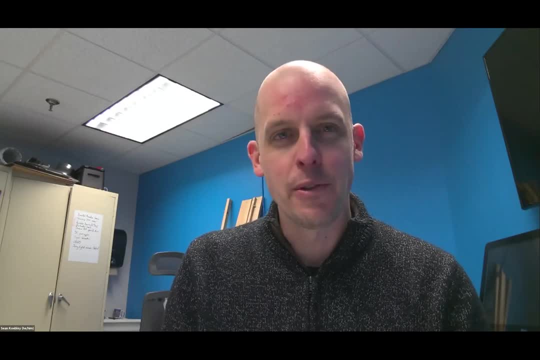 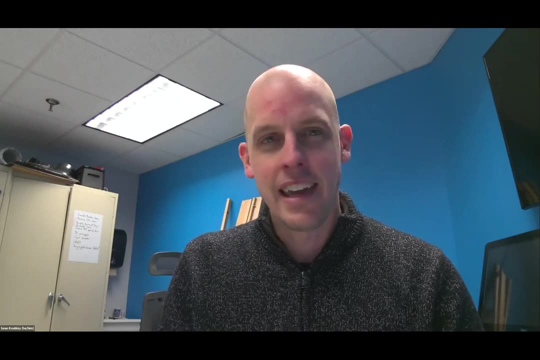 I'm very excited to be here today and share with you kind of this adventure that I recently went on with some of my research to dig into Bayesian statistics and maybe today I want to propose an alternative to the beloved, or perhaps hated, Bayesian statistics. I'm going to be talking 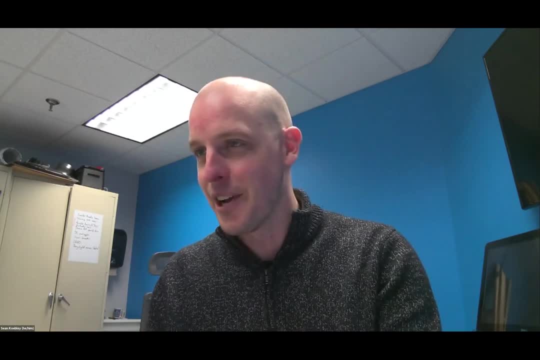 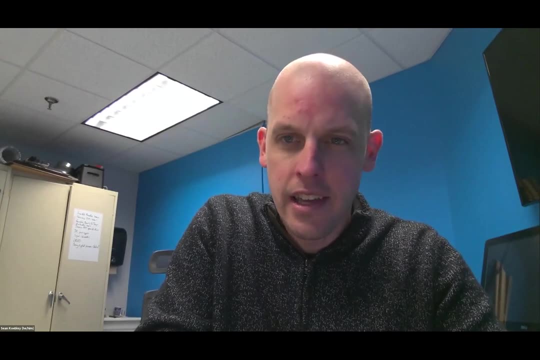 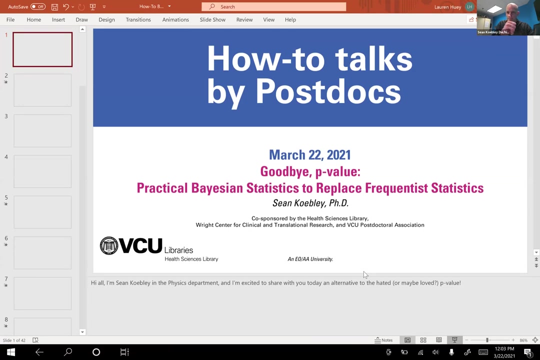 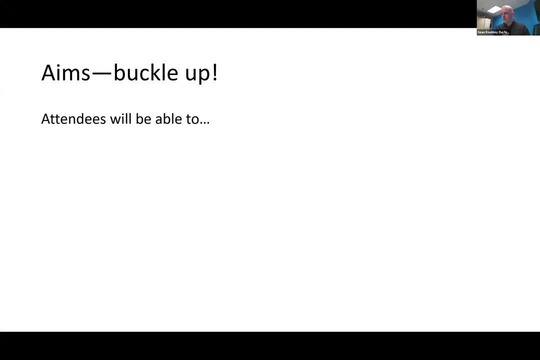 and see what you all think. So let's buckle up. So let me get my screen shared here and we can do this. All right, Are we good? Can we see that? Great, Okay, So maybe you've just. 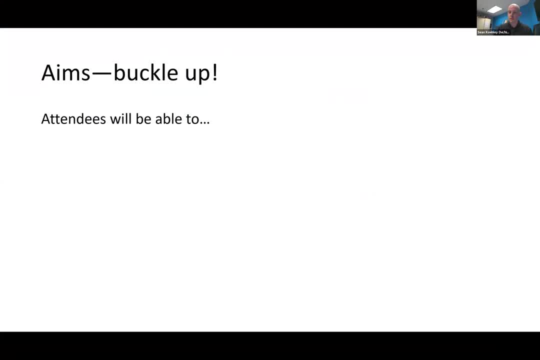